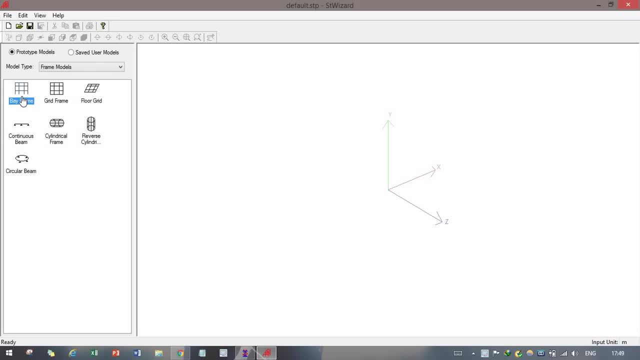 structure, then we have to create the geometry and then we have to create the. we have to click frame models. after clicking frame models, we have to click bay frame. after that, suppose we are having a length of 8 meter and the height of 8 meter and width of 10 meter and number of base base is nothing but your. 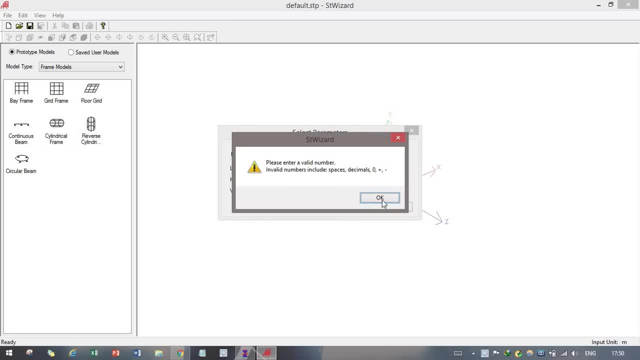 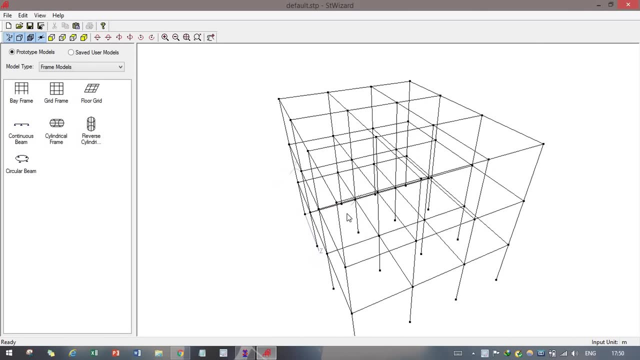 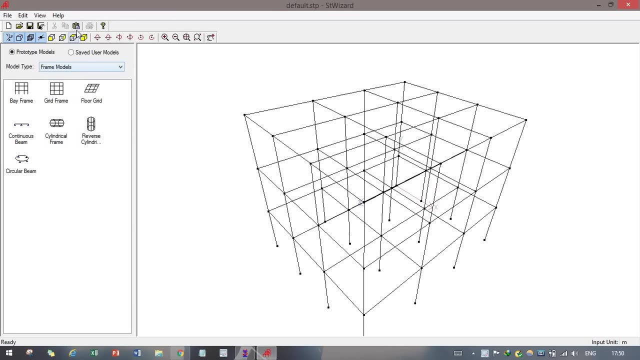 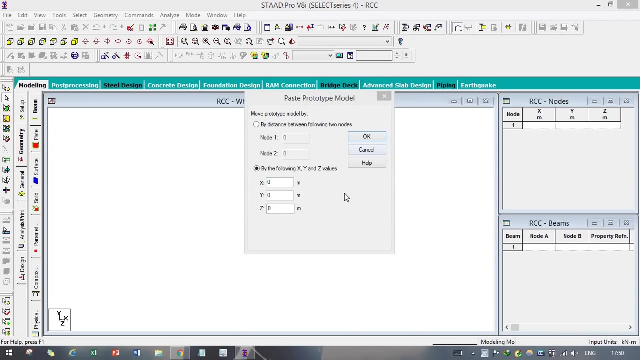 number of divisions along length and long, length and width and height, etc. after we have to click apply and, as you can see, our model has been created, we just need to deploy it. in our main page for the purpose, we have to click transfer model. okay, you can do this, you guys. this popup will come only for that. like how? 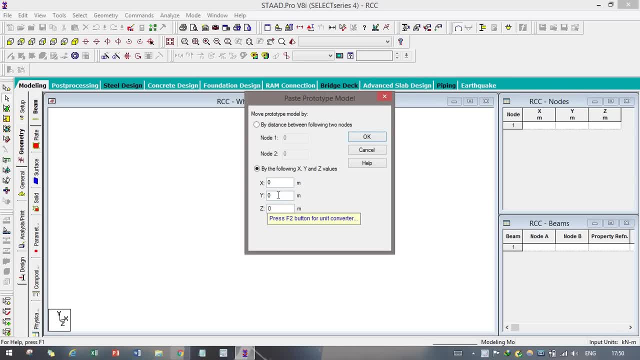 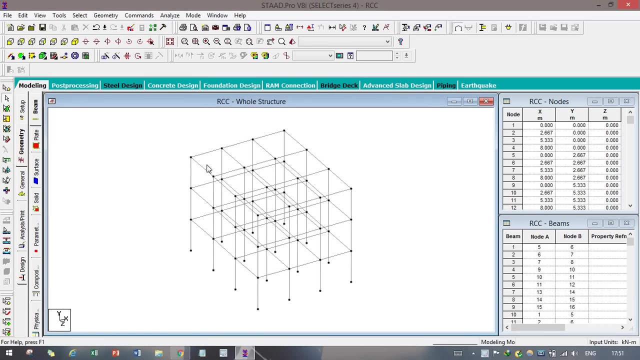 many distance above you want to. you want to deploy your frame model? okay, for the purpose, suppose we, if we are inputting so m5, value of 5 meter, or like 0 meter, 0 meter is like data, meet, datum point, so we are adding it as 0 meter. okay, the key will argue so. 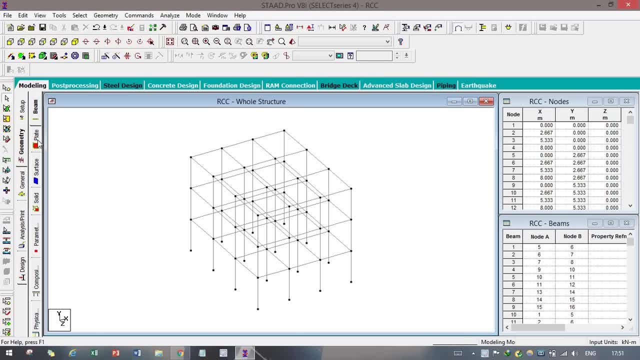 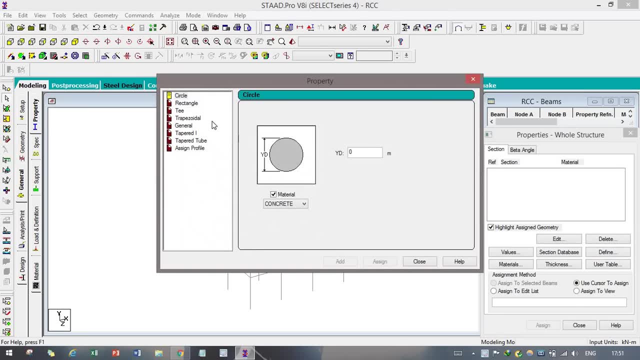 anik about category. we are, we just is cool, I'm logo frame Manalia for that general major, a jacket property. we have low category define cutting a number of properties we have to define before that. for that we have to click point 2, 5. suppose we having beam length. okay, rectangle is we are adding for beam length. 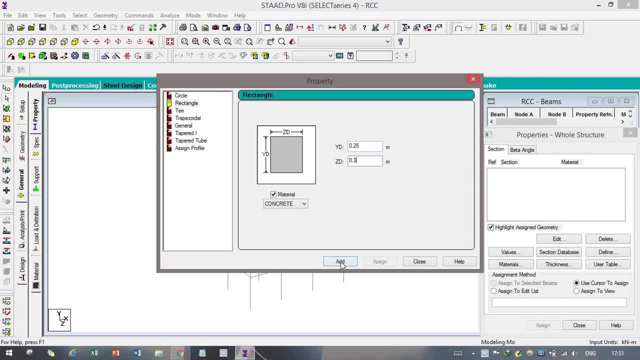 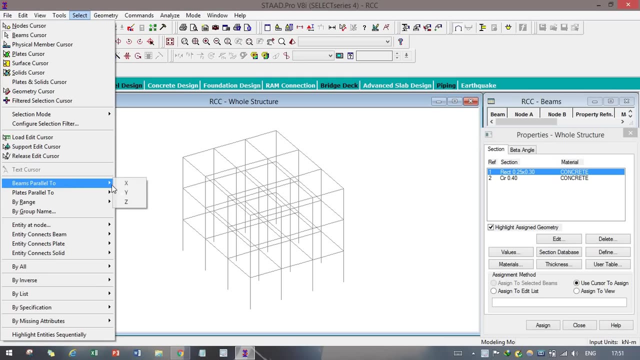 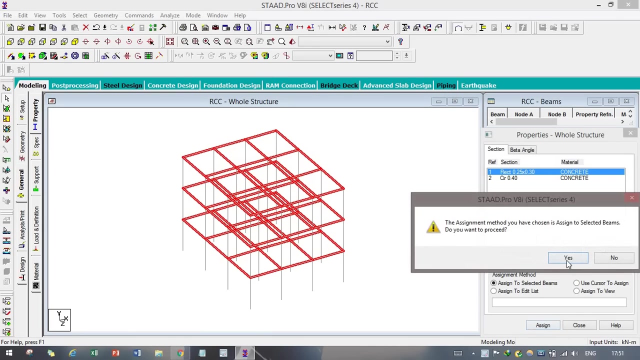 in our project. okay, after that, click OK. add after the circle, point 4, suppose this one is for column, we are X, adopting it's for rectangle, we have to click select beam parallel to X. select beam parallel to Z. okay, okay, it's done that you have to. 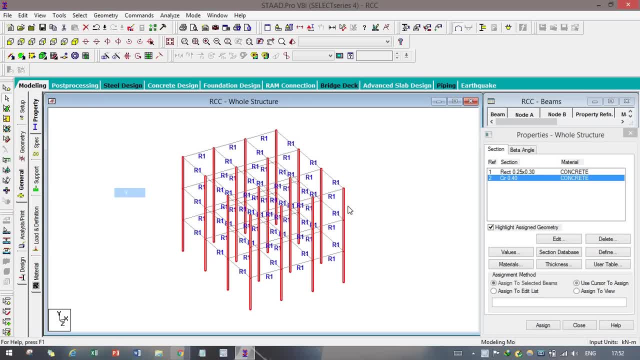 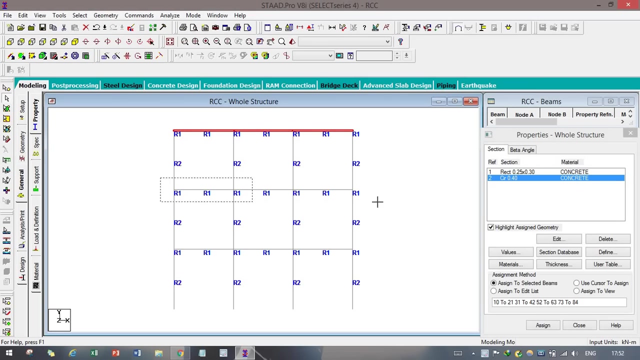 click circle. I have to click select beam parallel to Y, assign. okay, it's been assigned. after that we also have to create. we also have to create our slabs. so for that purpose we just need to, you just need to click. like that way these are front view. okay, so you can go to your isometric view also. after that we 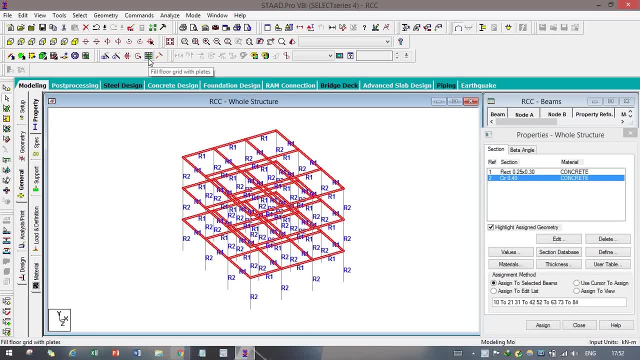 are creating our meshes, so for that we have to click this one, which will create what is the new plates has been created for that purpose: thickness, we have to give. thickness, we have to give. thickness, we have to give. density, we have to give to define, like we are having a floor thickness of 0.2, add okay. after that we 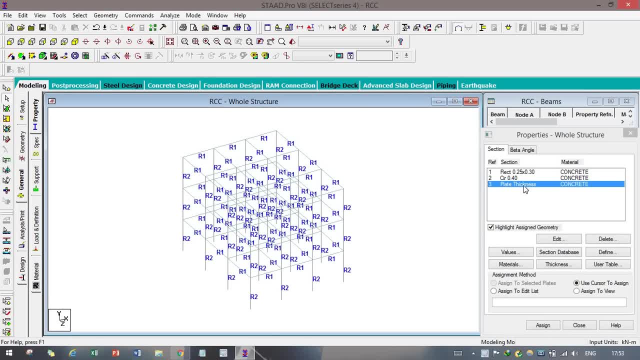 just need to apply those properties of plates into the whole model. so for that purpose we have to click plate cursor and click whole area only plates will be get selected. after that plates thickness is also selected. if they assign it. okay, it has been assigned. after that you have to go: support, okay, support, suppose. 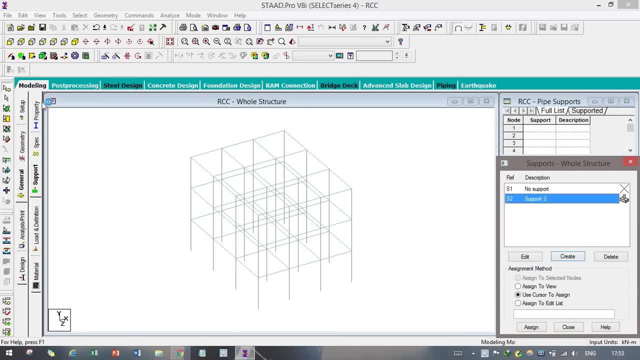 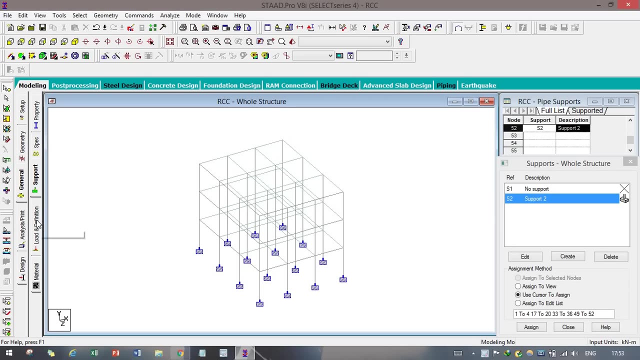 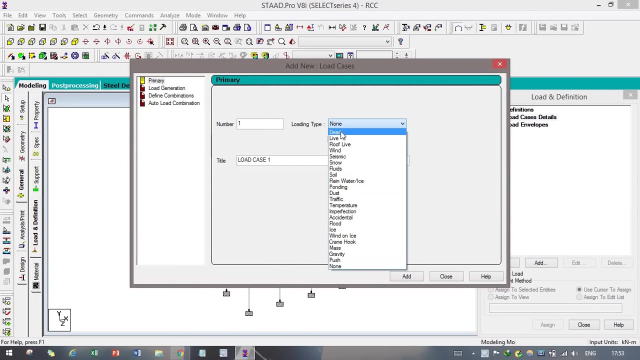 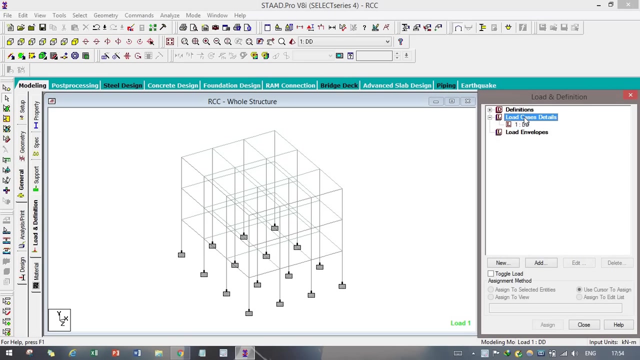 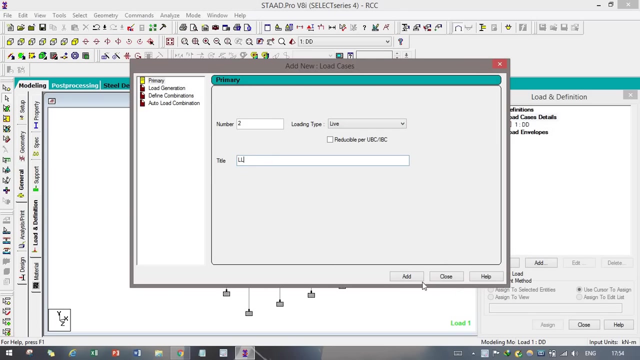 we are having all the fixed supports and have to go front view, then drag down the all the nodes for support purpose. okay, after that have to go isometric view and after that we have to click load and definitions. in load and definition: okay, We will have dead load for loads which are due to your self weight and active members, etc. Okay, Another load we have to create, this one is live load. This is LL. Okay, In dead load we are having self weight of the structure. Okay, 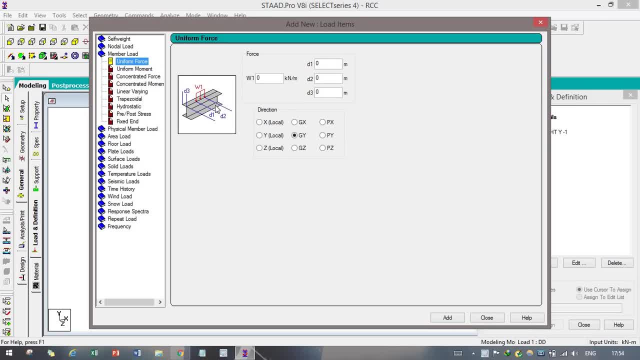 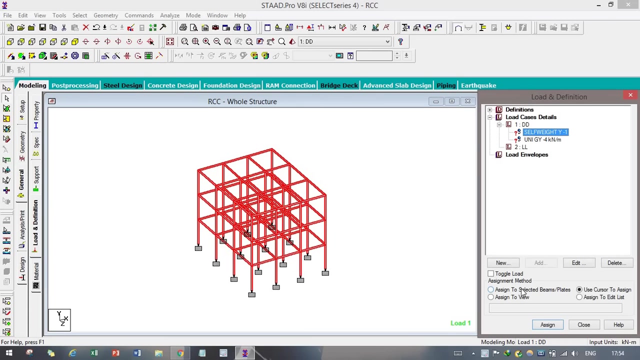 Okay, Simply adding. add After that your own member weights, which are already like concrete beams, which will be its weight. So for that, my whole dead load is 4 kN. Let me turn, add After that I have to assign it. Assign to view: Cause it: self weight, Self weight. will be done for me. 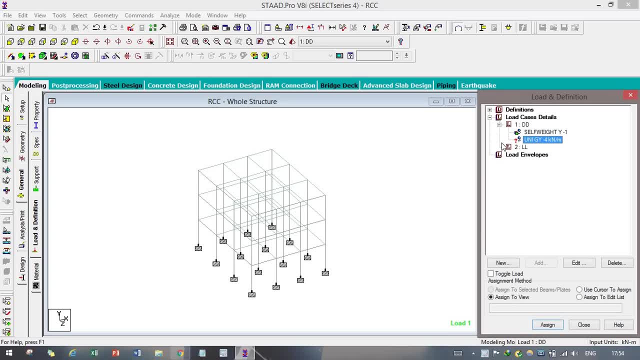 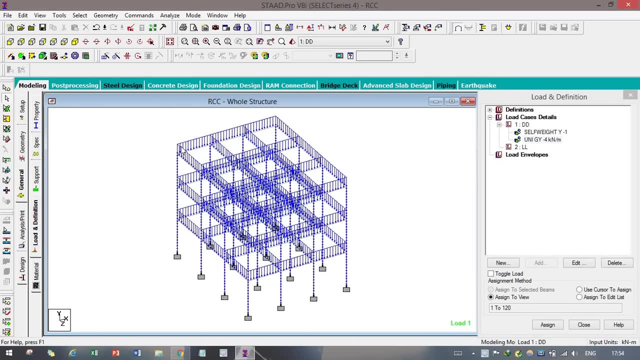 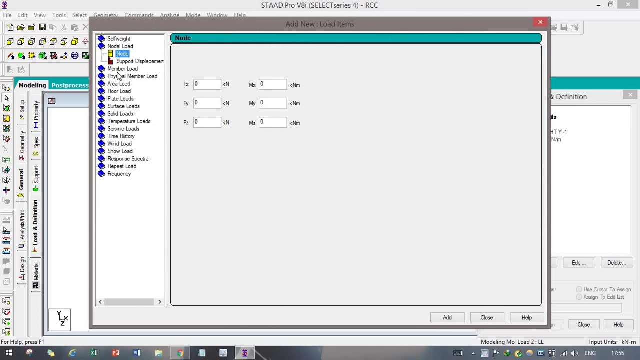 For whole member So that we have to click dead load for whole member. In case of, as you can see, all are UDL, Like beam's length, which is equal to the weight, will automatically come in dead load. After that live load Add, You have to click on member load. 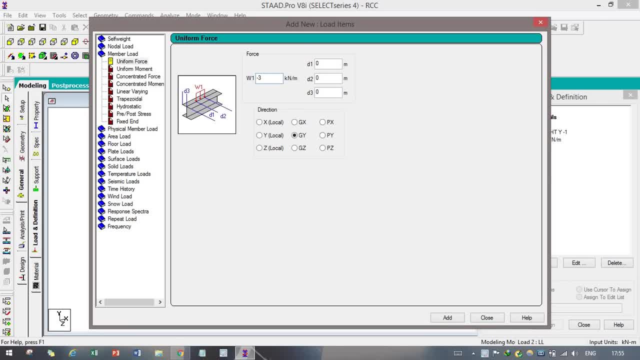 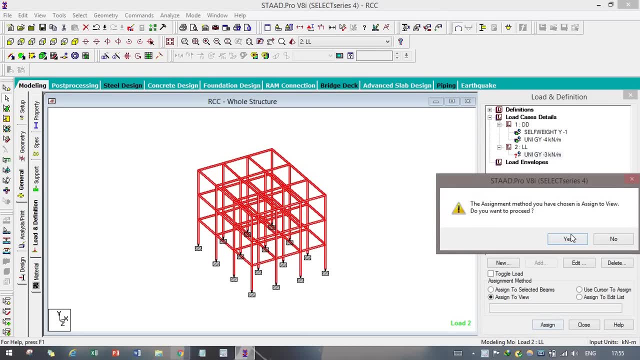 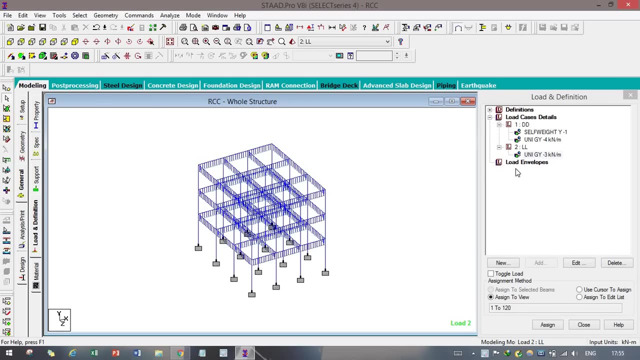 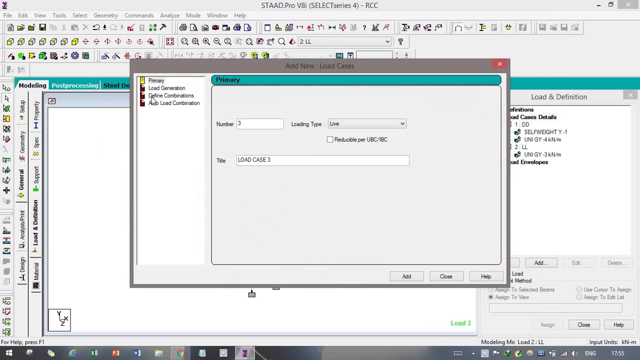 Suppose: live load, we are considering 3. Okay, Then add: You have to click whole surface. Then assign to view. Okay, All has been done. If we are adding extra safety, Then what we will need have to do, We just have to create combinations. Okay, Load combinations. 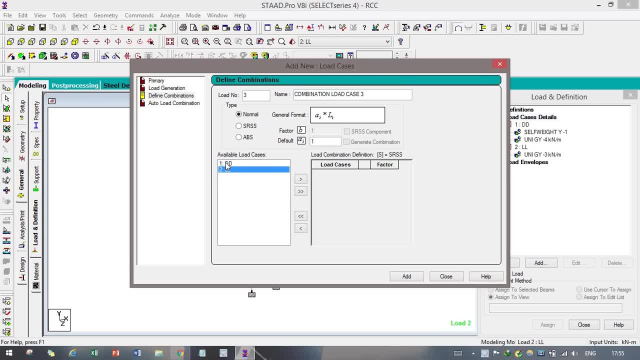 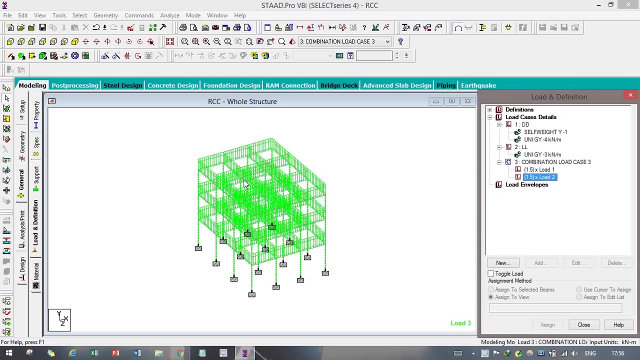 In design: the factor of safety. So this one is factor of safety, Okay, So suppose we have predefined one. We can do 1.5x1.5 with every load. Okay, For better security of the structure. Add, You will get combination load according to you If you will see all the loads combined. Okay, All done. After that we have to go analysis and print. 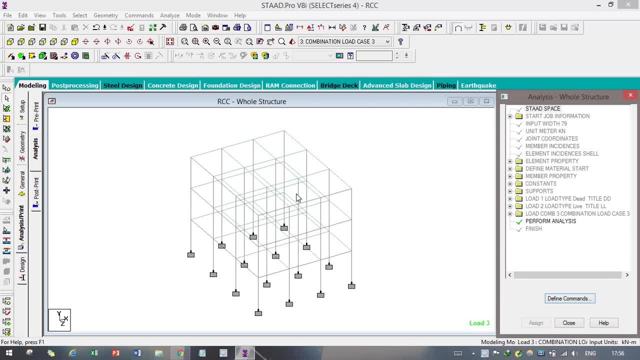 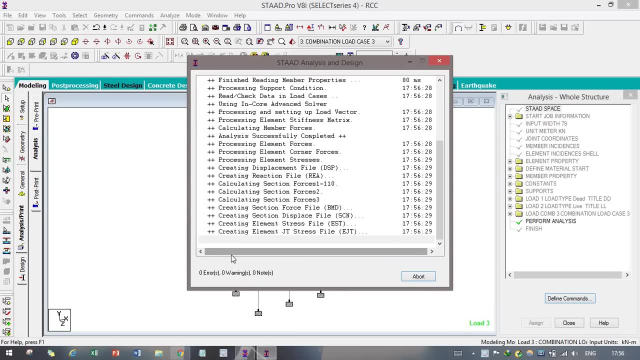 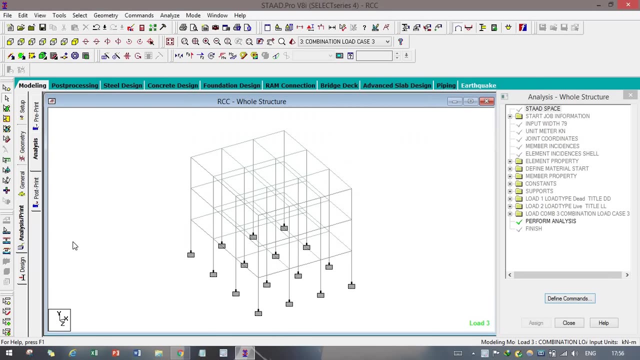 Let's first check whether we have done anything wrong or not. Nothing else? Okay, Have to go analyze, Run, analysis, Save. We will check whether, whatever we have done, Are all these things are correct or not. Okay, Then after that we will go design. 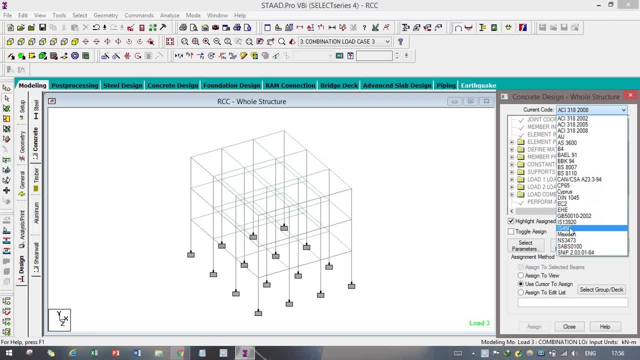 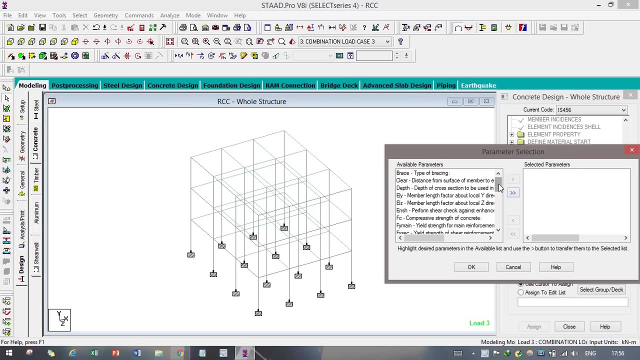 We have to click complete design. We have to select our code. After that we will have to do, We will have to set our parameters. Select parameters, Like all parameters you can assume as your requirement of structure. Right now we are not assuming all these things. We are simply adding clear cover and comprehensive strength of the concrete and real strength of the main reinforcement. 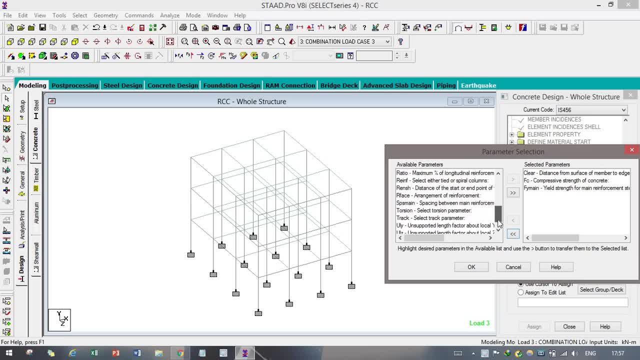 That's all. You can further add your parameters Like torsion for torsion purpose, And track And width purpose- Unsupported length. On basis of that, you can select your own basis Depending upon your structure. Right now, we are simply adding all these three parameters only. 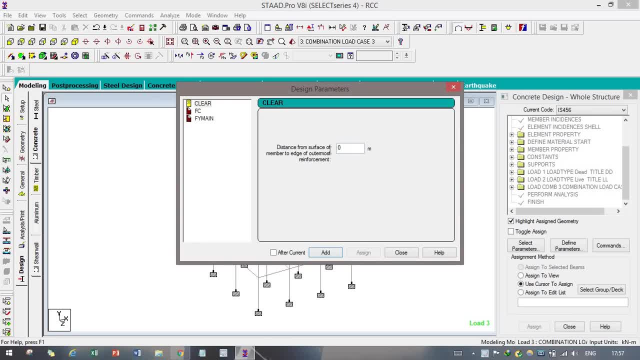 Okay, We have to define it For the defining purpose, Suppose we are having clear cover of 25 mm. So what we will have to do, We have to write it in meter, We have to click add After that concrete: Suppose we are having M20 grade concrete. 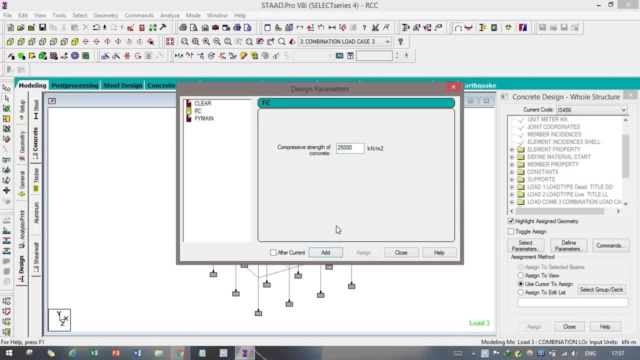 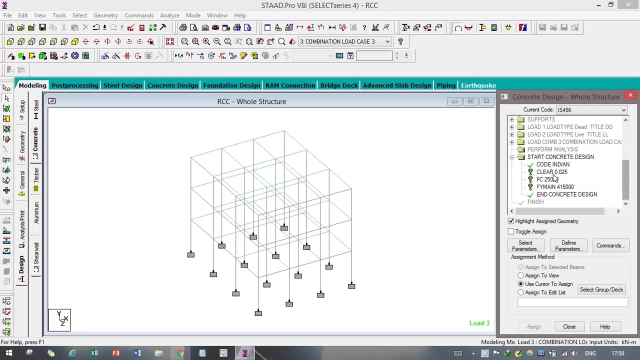 Okay, M20 grade concrete. So we will have to click on add. After that, for main purpose, We are having mile strength of real strength: 415.. Okay, After that we will have to Simply assign it. Okay, Assign to view. 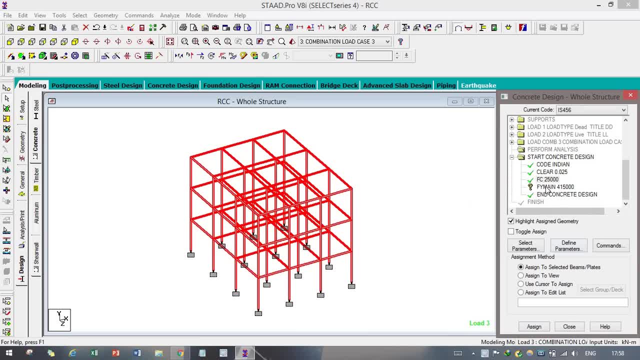 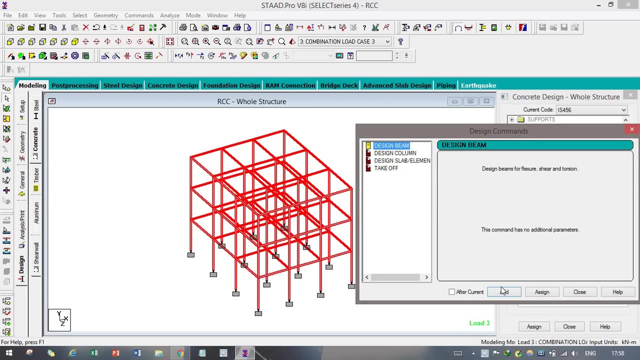 Assign to view Assign, Because these are concrete and steel properties. Okay, So these are, These are concrete and steel properties. After that, we will have to also Also design, And just adding: Designing of beam, Designing of column. 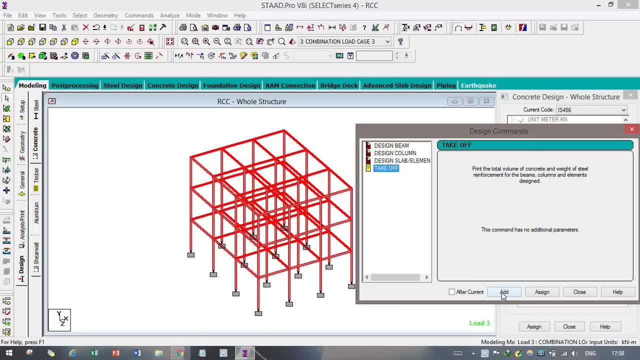 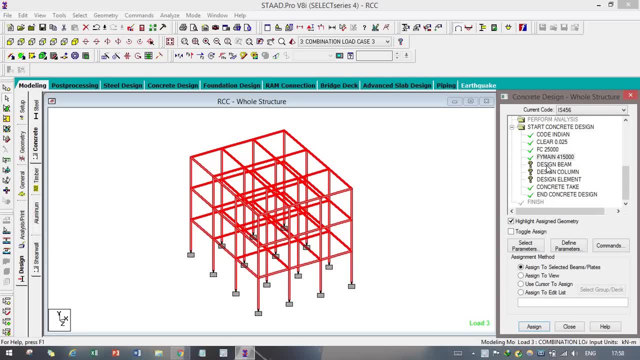 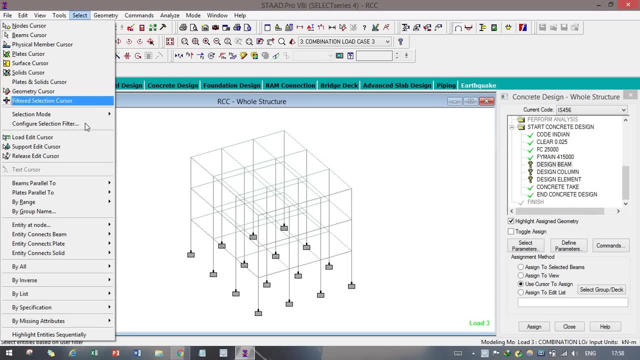 Designing of slab And takeoff For all, summarizing the concrete length and volume of steel required, and all Okay. so you just have to click design beam: okay, design beam for design beam, which we only have to select. beams only okay, okay, okay, design column select. 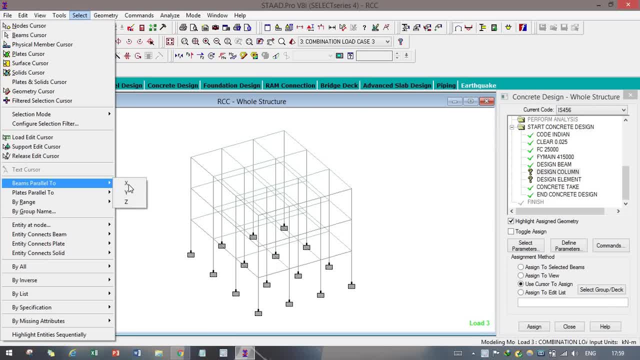 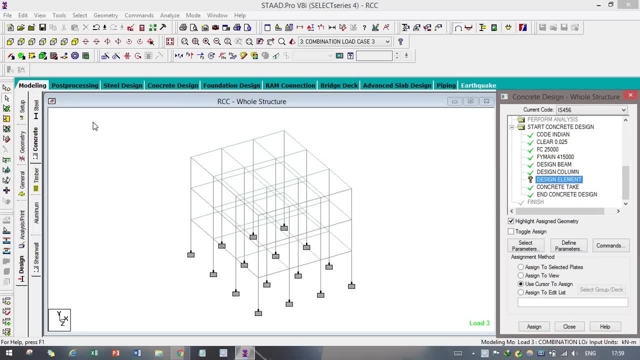 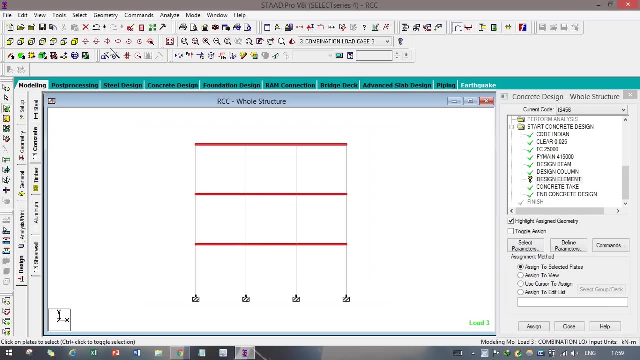 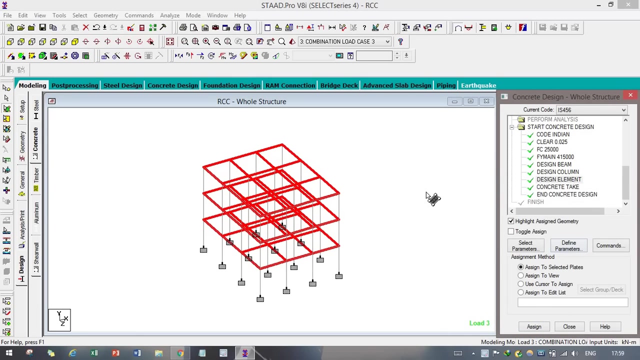 be parallel to x, only columns. we are selected in design element. we will see. simply have to go click. we will have to click plate cursor. after that we have to drag down all the whole structure. only plates will get selected. and after that we are designing the slab. just to assign it all has been done. after that we have to. 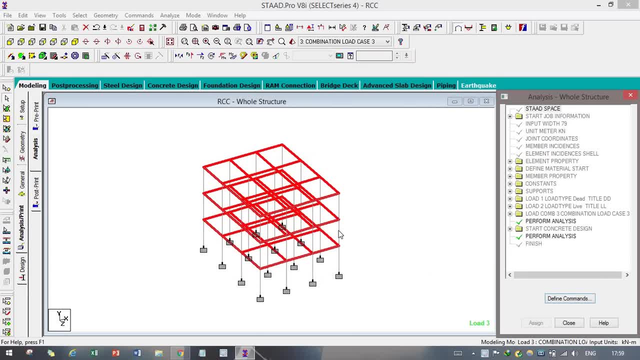 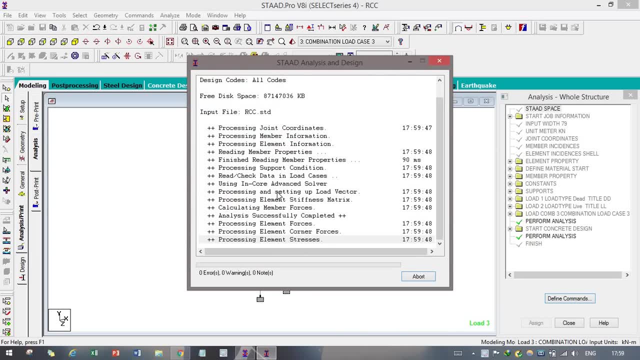 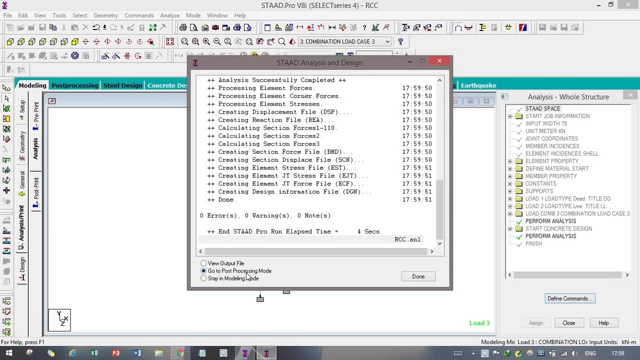 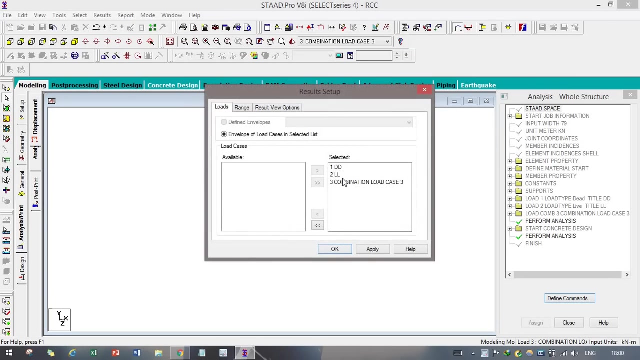 simply go analyze this. no print analysis. add close. okay, after that we have to analyze run, analyze, run. okay, as you can see, all no error is in our. they are in our structure. we have to go post present mode for our output file and further details. we need to check. 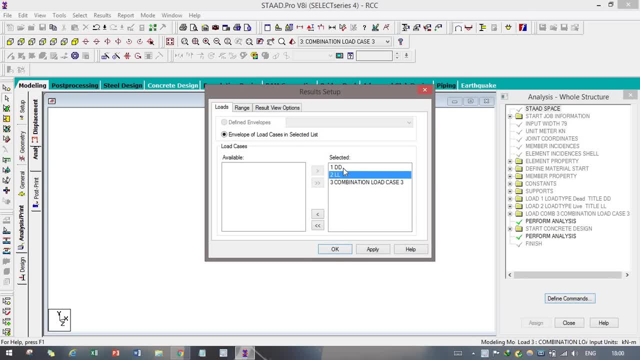 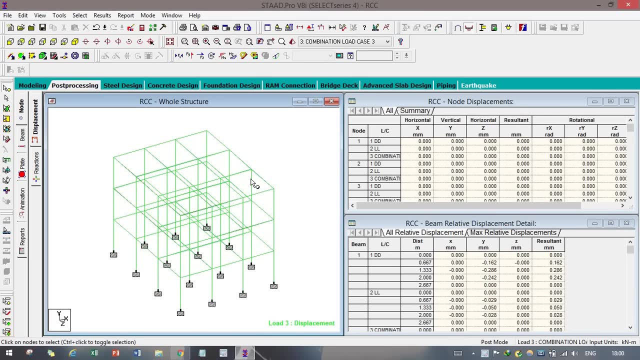 we, we are having all our details with combining all loads. okay, now you can see, by pressing the control button and mouse scrolling we can simply check our deflections and our moment in m z direction, moment in moment in bending, moment in y direction, then boom bending moment in the x direction. okay, 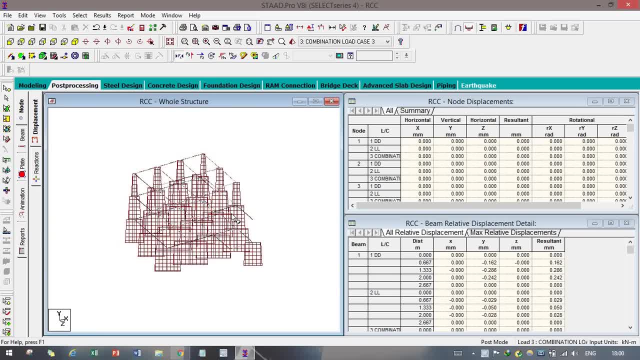 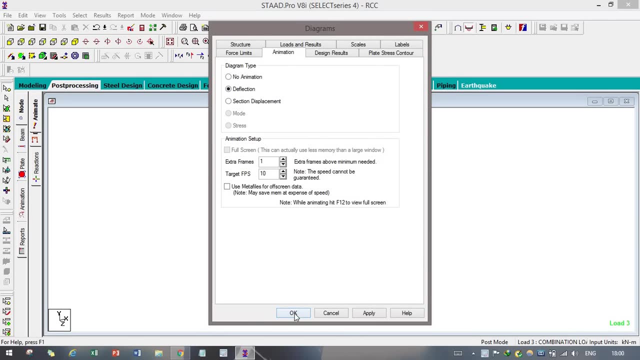 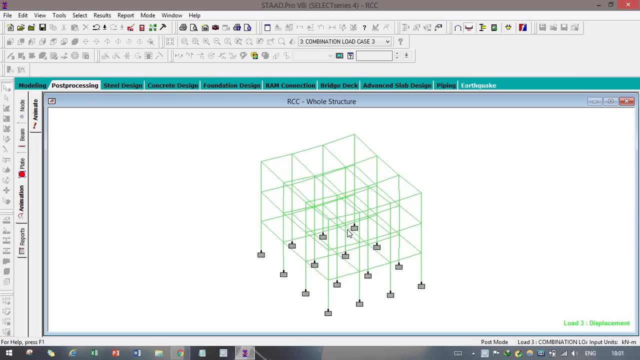 then share force. all are the shear forces. you can simply uh in and out for a better understanding by by pressing the control button and mouse scrolling button. okay, okay, right now i just want to show you guys animations of the structure, how structure will behave under such load. you can see structure will behave like this way under the certain load you can. 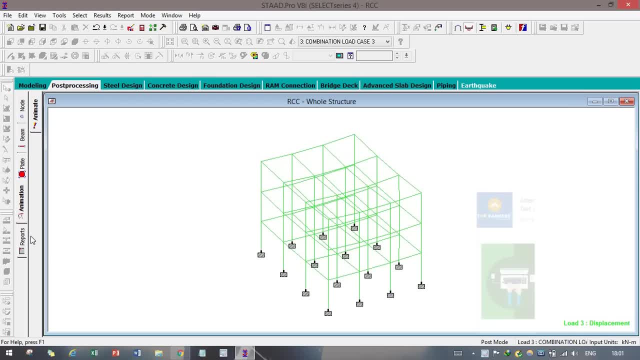 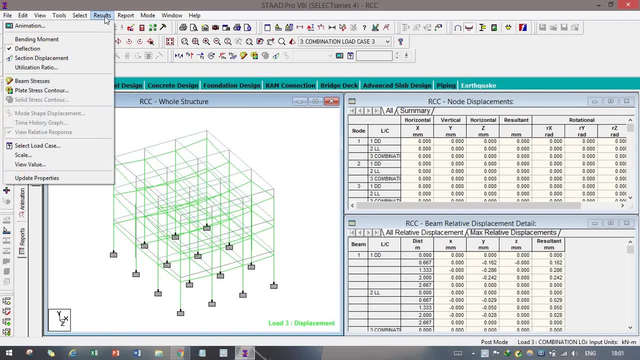 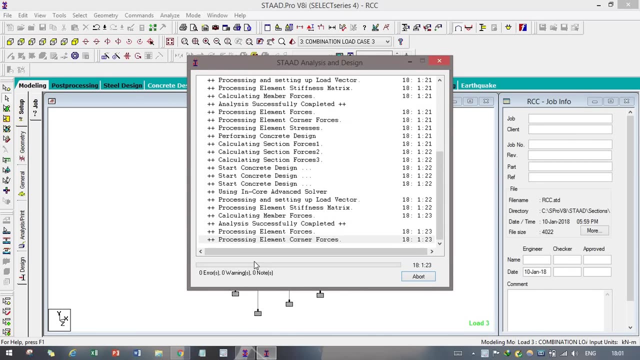 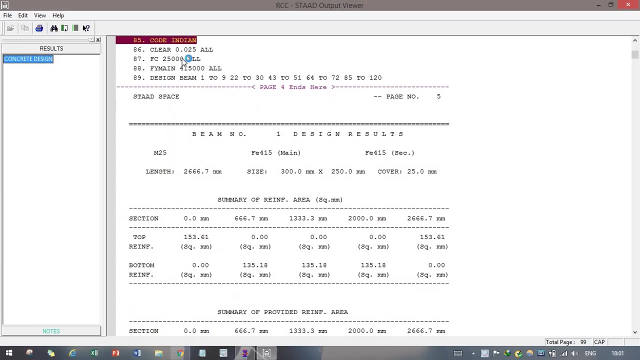 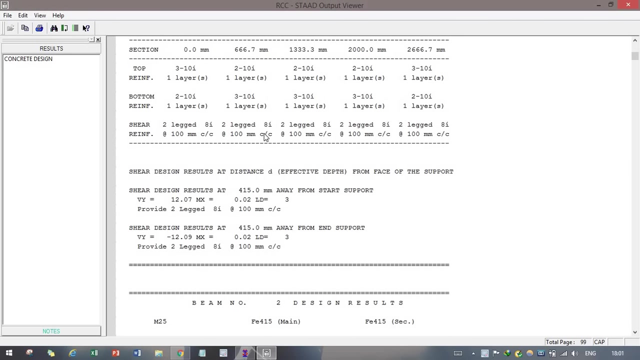 understand all the things after that. if you want to understand all the things after that, if you want to have your report, like suppose you, you want to have your final sheets, having all output file. okay, so for that purpose you can go. complete design. you can see each and every beam has been designed in proper way and